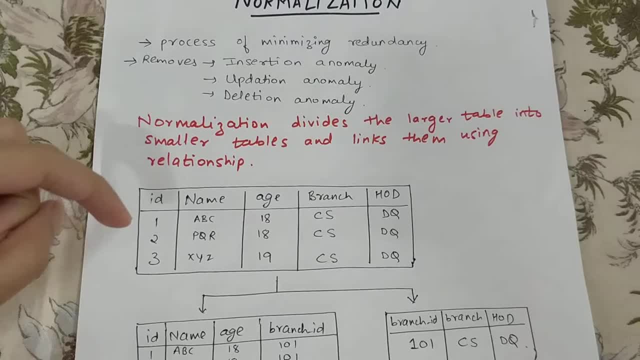 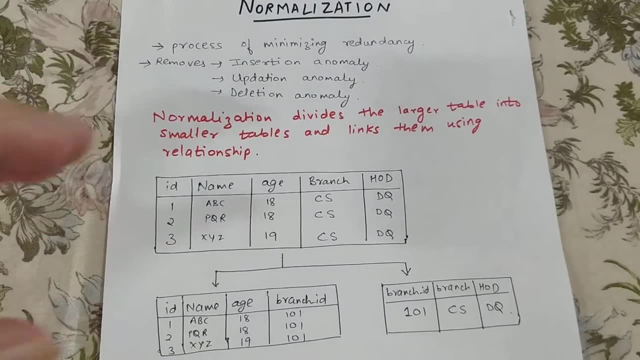 where all the data is repeated every time. So normalization basically removes these repeated data. All the information is in just one single table, which is wrong. So normalization divides that big table into small tables and links them. That is what normalization does. So, as you can, 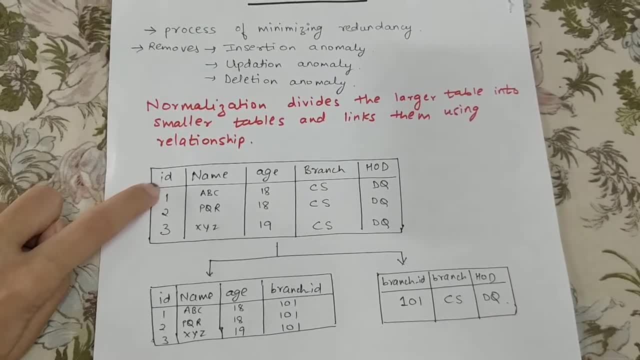 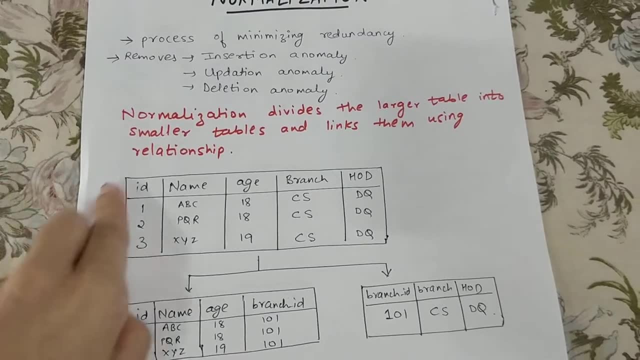 see this table. this is a student table, So here there is an ID name, age and the branch which the student belongs to and HOD of the branch. Okay, so this is one table, But, as you can see, 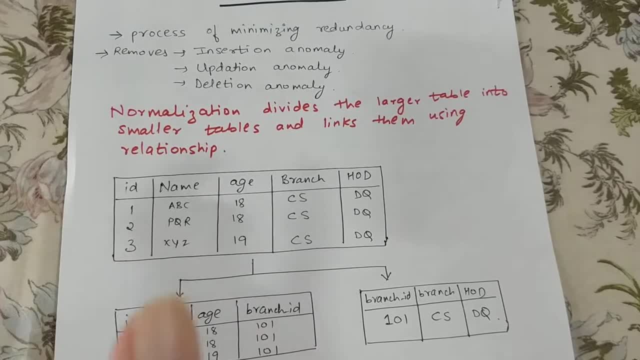 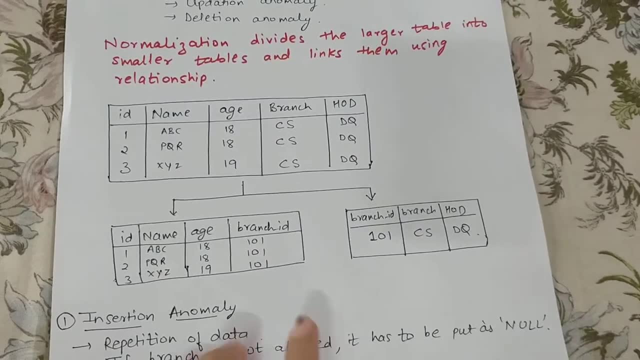 this one table actually is equivalent to two tables, isn't it? One is the student table and the other is the branch table. So in normalization we'll divide into two tables. Like this is one student table, ID name, age. 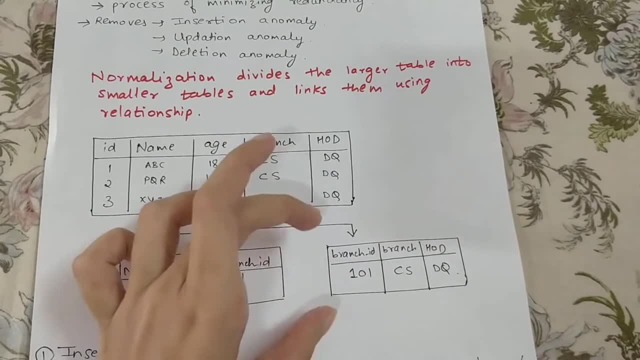 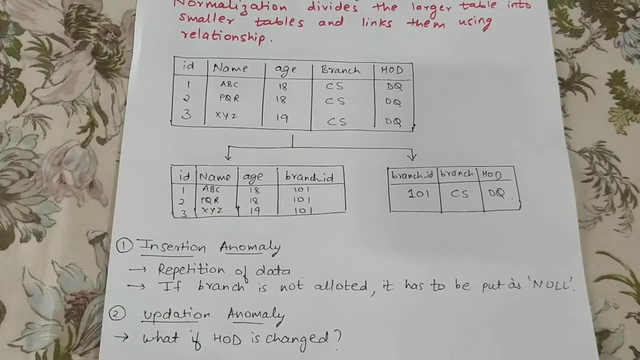 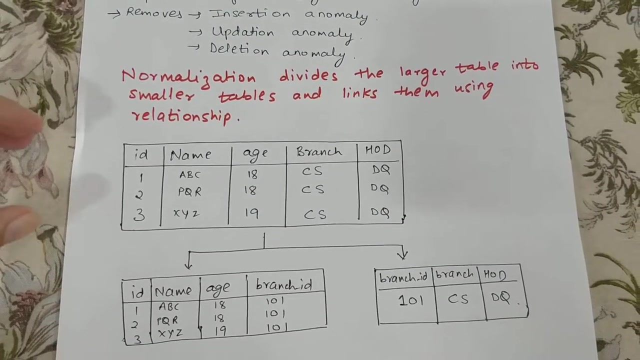 and branch ID And there will be another branch table which is branch ID, branch and HOD. Now, why we do this? we'll understand it when we understand these anomalies. Okay, but let's understand. but we'll understood that normalization is basically converting one big table into smaller tables. 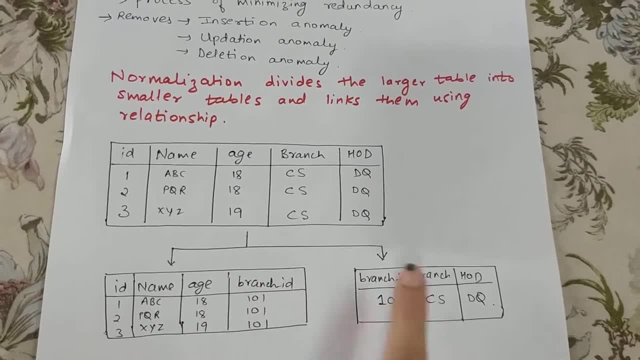 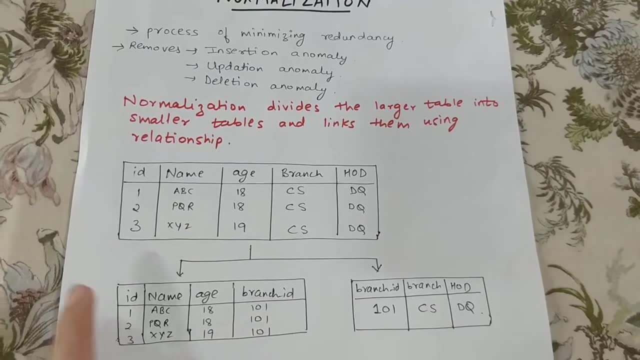 and linking them. Okay, As you can see, we are linking these two tables through through this foreign key. as you can see, branch ID. Branch ID is over here also, branch ID is over here also and in that way, the two tables are linked together. 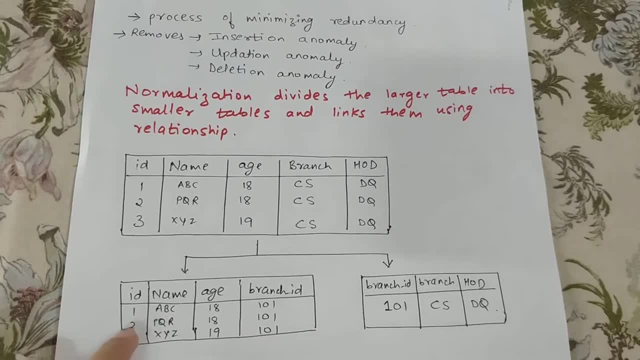 And if you want to know what is the branch which ID No 1 belongs to, So we'll go from. here is ID No 1.. Name: age branch ID number one. Name: age branch ID number one is Randy facade. age image speech numerous. 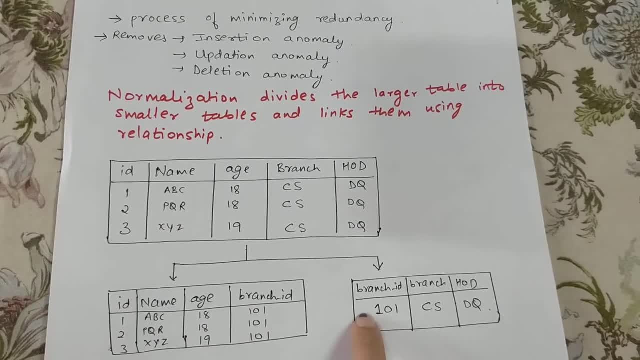 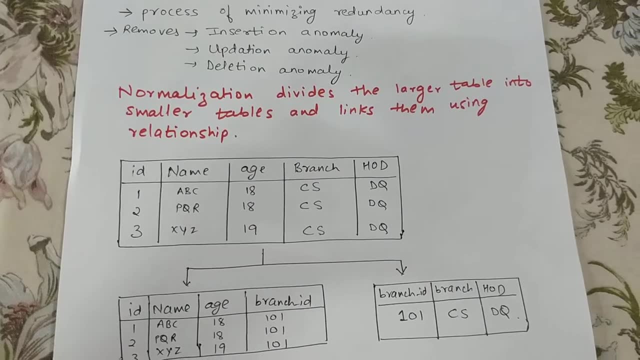 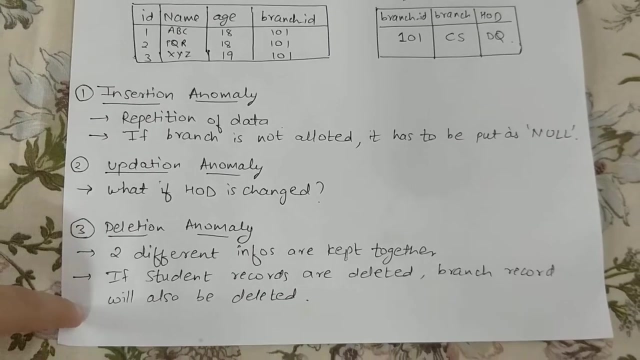 is 101, so we'll check in the branch table. so what is 101 or what is a branch for 101, CS? so we'll understand that the branch for ID number one is CS. okay, now we understand these three anomalies. these three anomalies occur when the 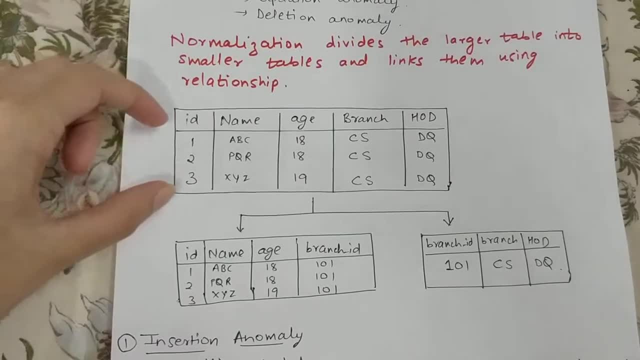 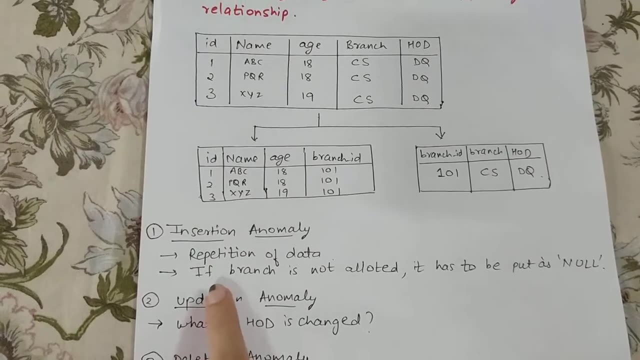 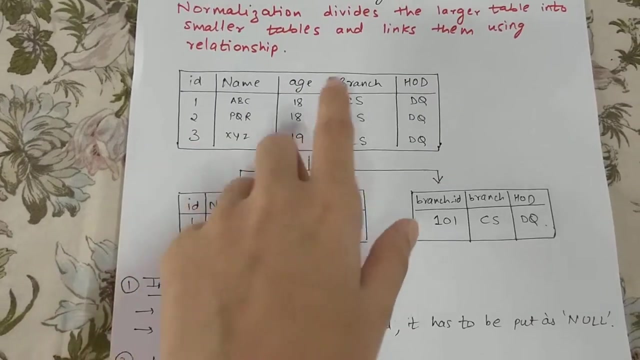 table is not in the normalized form. when, basically, the table is a bigger, the one the big table. okay, when it is a big table. so this over here. so now, the first angle which we are going to understand is insertion anomaly. so in insertion, animal anomaly, repetition of data is there, as you can already see, as already. 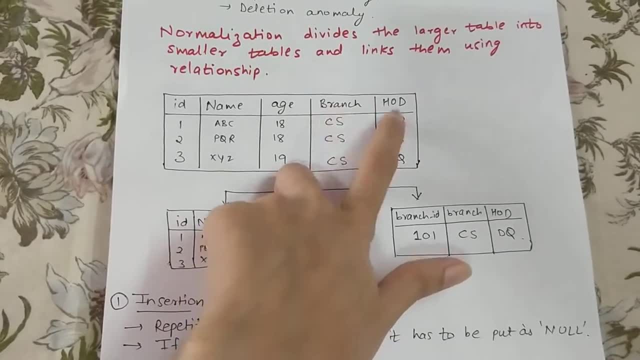 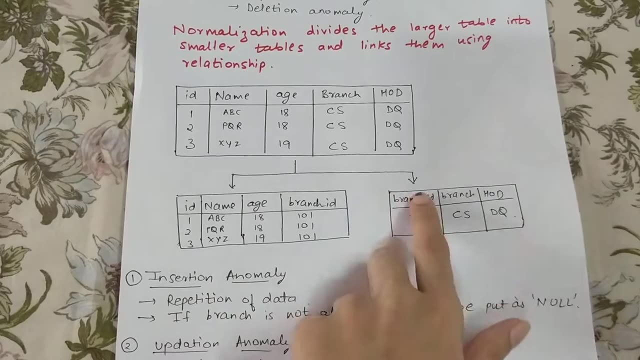 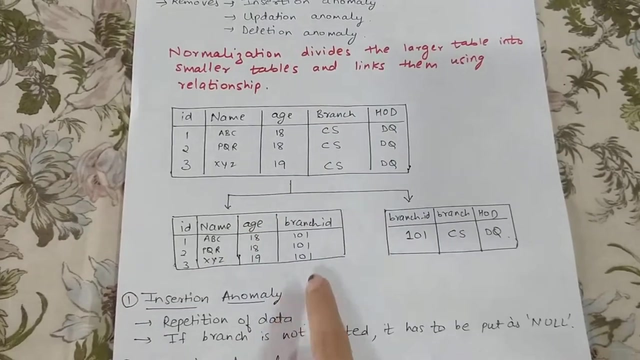 said here, the branch information, HOD information, is repeated every single time now, but when it is in the normalized form, this anomaly is removed. how, as you can see, you are not repeating CS and- sorry, branch and HOD information every single time. instead, you're just writing the branch ID over here. okay, 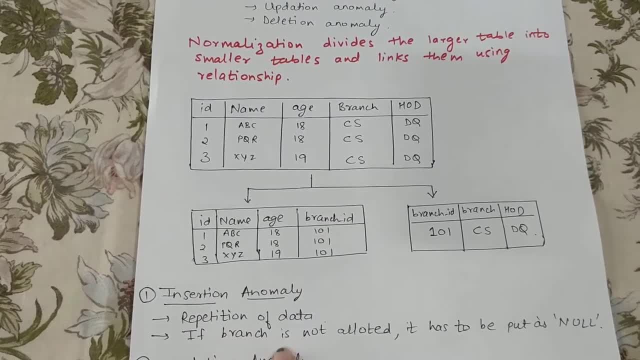 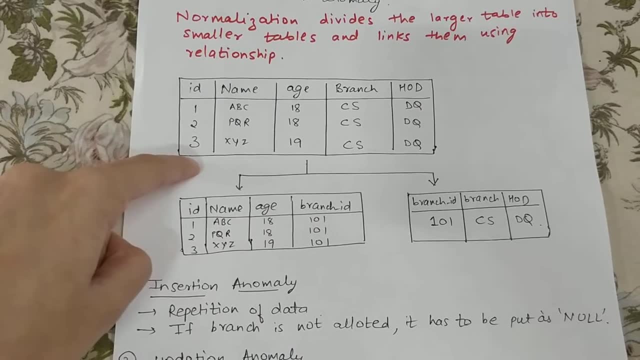 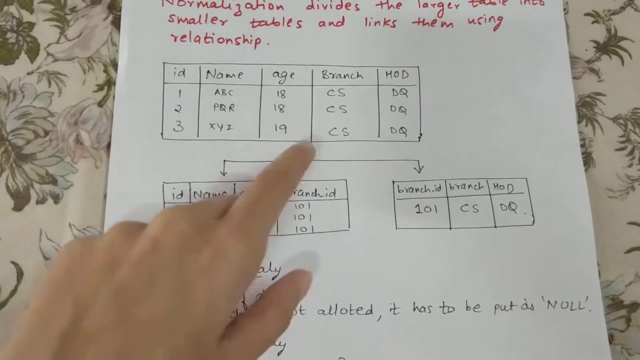 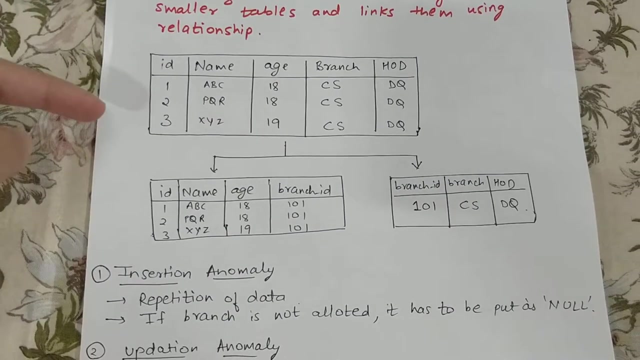 okay. now if branch is not allotted to one students, for example, say, you want to insert a new idea here and the branch for that particular ID is not allotted yet. so you have to either keep it null, or you cannot or not insert that ID in the table. that is what. 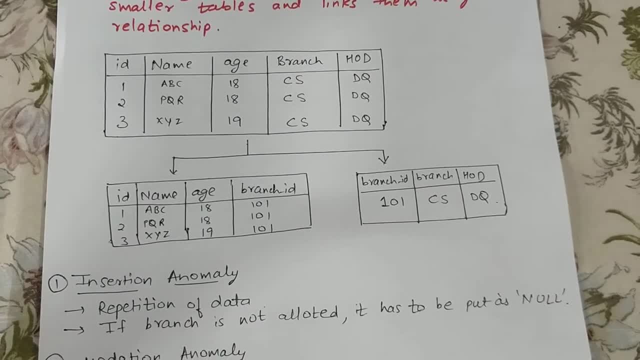 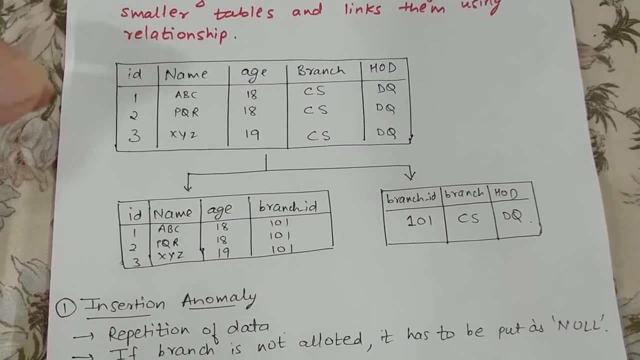 insertion anomaly is all about. now let's say the branch called the branch is allotted to it. now that is how the is hard. and now let's say the branch calls the branch to the 그럴 that acknowledge has has a restriction that you cannot not insert a null value over there. so 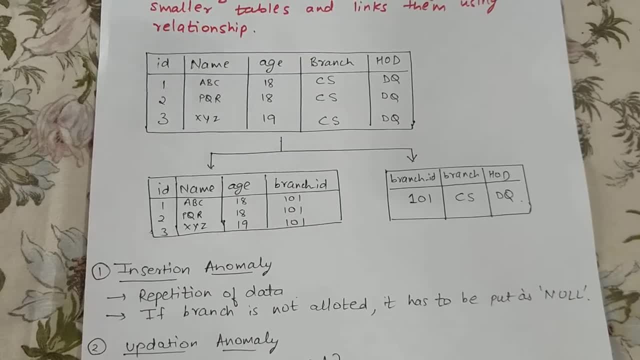 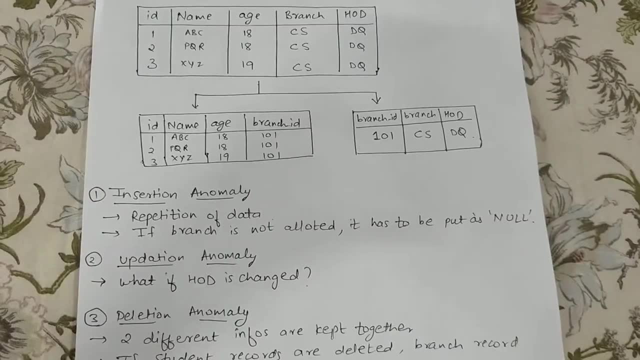 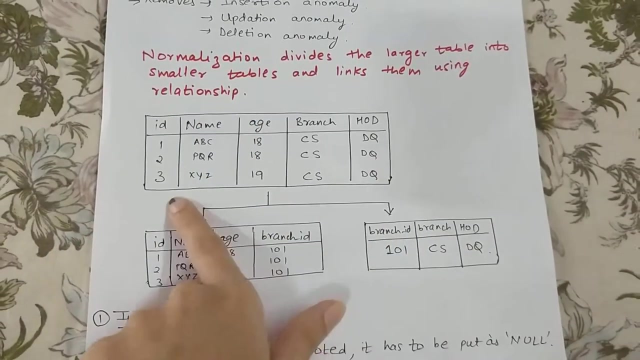 you will not. you will not be able to insert that IDs information at all, and that is what. what insertion anomaly is all about. okay, second is updation anomaly. now, what if HOD is changed? now suppose this table is over here. this is not. this is not the normalized form. now, for example, the HOD for the branch CS is: 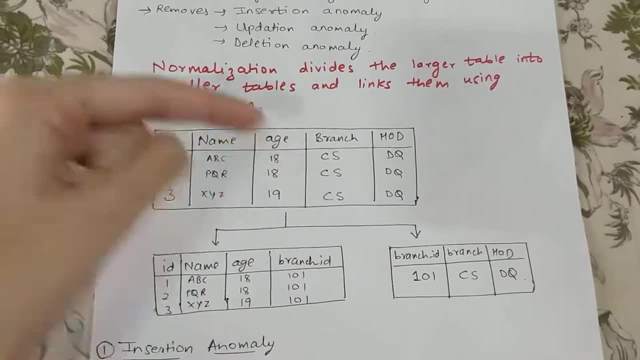 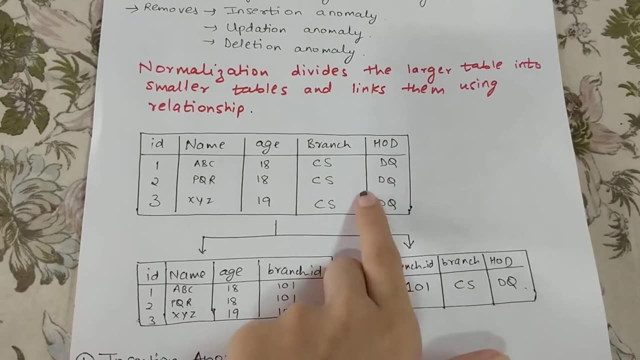 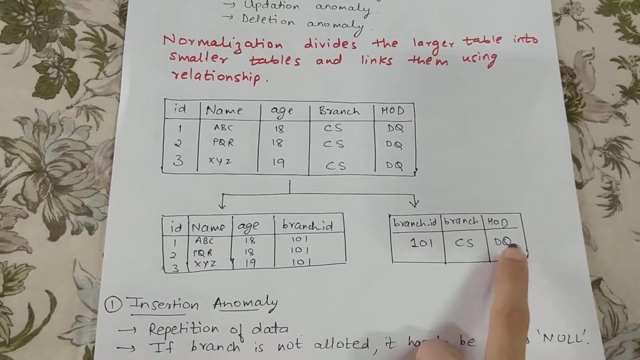 changed to say a- B. now you will have to update every single column over here and you have to change DQ to a B. every single row you have to change. but if it was in a normalized form, you you would have to only change it over here once. 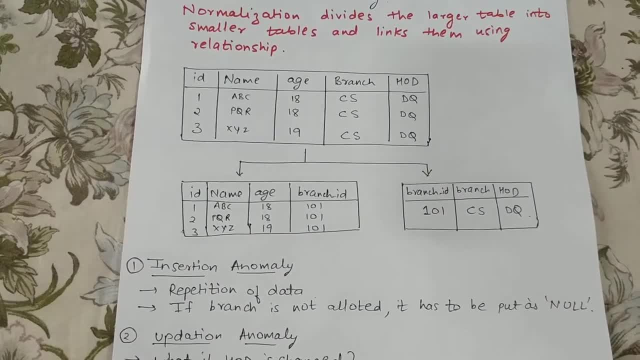 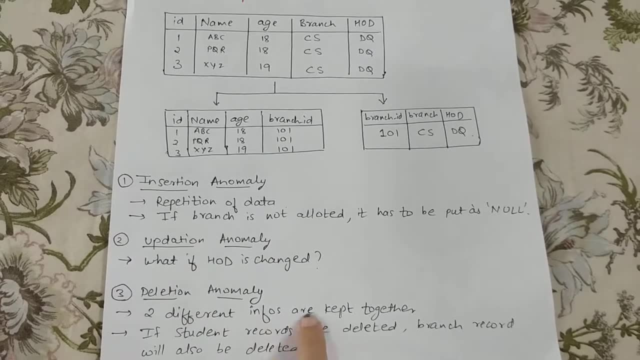 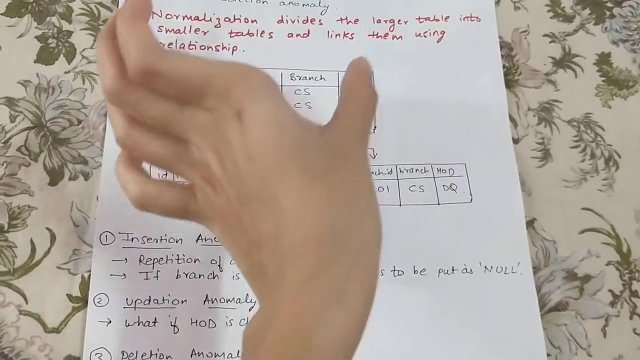 and that is how updation and she anomaly is removed. okay, next anomaly is deletion anomaly. so basically, two different informations are kept together as already, as I already said that two informations- one is of the student and branch- everything is in one single table, so two different formations is in one.